is: we're going to do this in steps. So what we're going to do is: we're going to do this in steps. So we're going to do this in steps. So what we're going to do is: we're going to do this in steps, So. 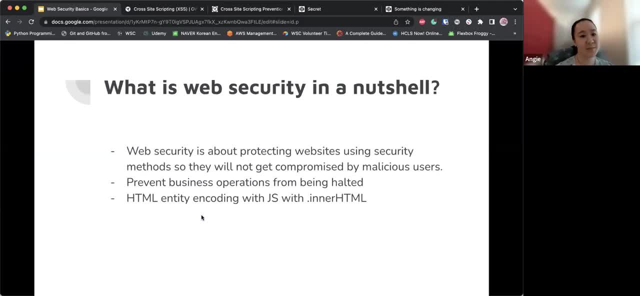 there we go- A web vulnerability. There we go A web vulnerability. It, you know it can prevent business operations from being halted, And a way of using like web security methods would be HTML entity encoding with JavaScript, with inner HTML, And I'll get into that when we are further. 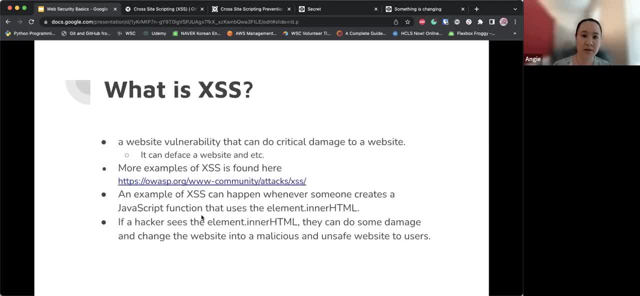 along. So I wanted to first talk about cross-site scripting before we get into the HTML encoding. It'll make more sense when we do this, So I'm going to do this in steps, like a little hands-on activity towards the end. so i'm, when i think of cross-site scripting, it also 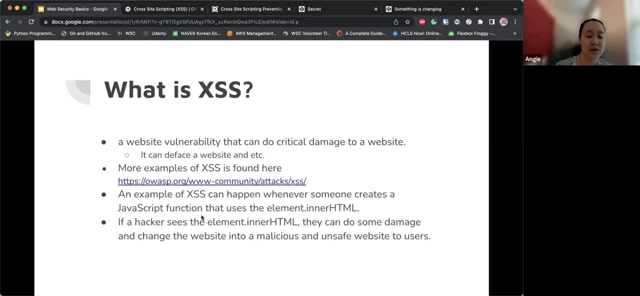 is known as xss and it can do critical damage to a website, so it can deface a website. there's so many different things that cross-site scripting can do and there's a lot of examples that are um found in this link here by OWASP, and when you do click on that link, let me see here. 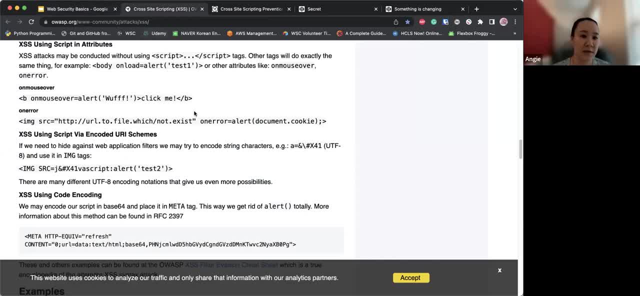 yeah, when you click on the link here, it gives different types of examples of what cross-site scripting looks like. so it's typically with the script tag and then within the script tag you have things like on mouseover events, um alerts, click me on. excuse me, not on. yeah, on error, i don't know why i was thinking it was one error on error and 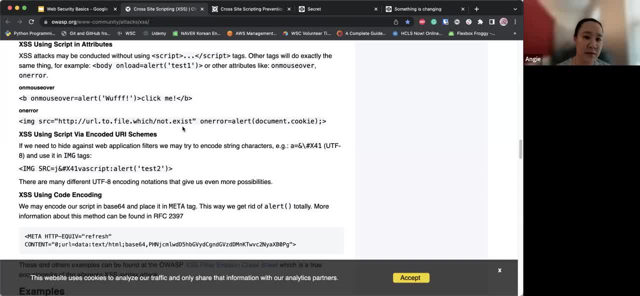 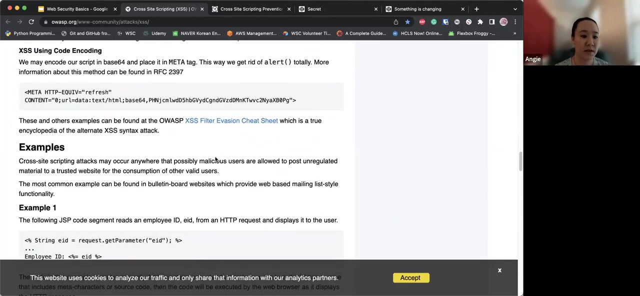 you have the image source and you have a url and then you have it on- yeah, on error alert here- and that can be malicious because, again, if you can put anything inside the tags, that can cause critical damage to a website, even with um encoded, uri schemes, etc. and there's there's a lot of different examples that i'm not going to go through, but 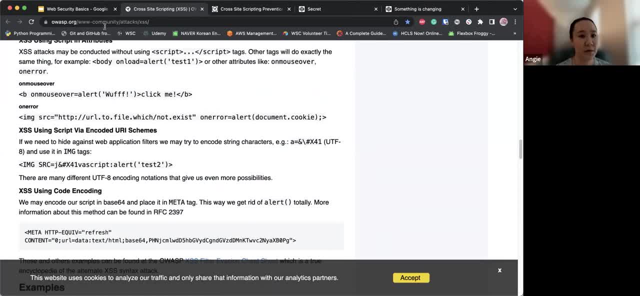 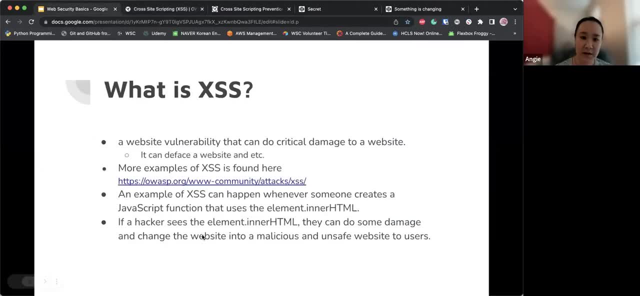 these are just a few of what we'll be dealing with when it comes to the html encoding, and i was also mentioning that whenever you see something with elementhtml, elementinnerhtml, it can be malicious because you can put whatever. like i said, you can put whatever you want inside. 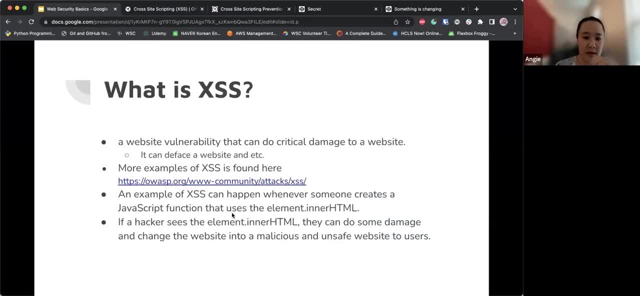 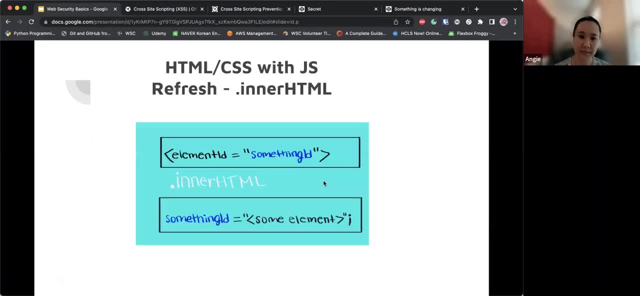 there as an attacker. when you think about what the attacker can do, they can put in different types of payloads and whatnot in that script and we don't want that to happen. so i made a little illustration for those who have not had, like, any familiarity with html, css and javascript, because it is a web security basics. 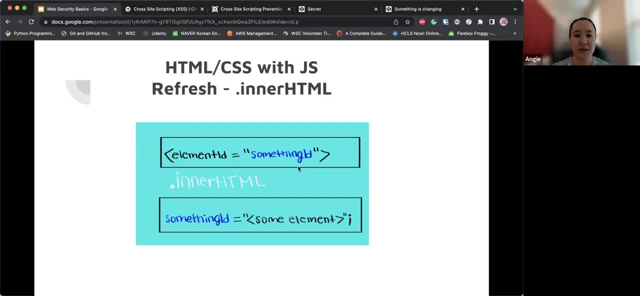 webinar today. so, if you don't know much about html, there's something called like an element id and there's, and then you can assign it to some text. and when you use innerhml- this is with javascript- okay, dot inner html- you can assign that id, that text there that you have assigned to the hml element. 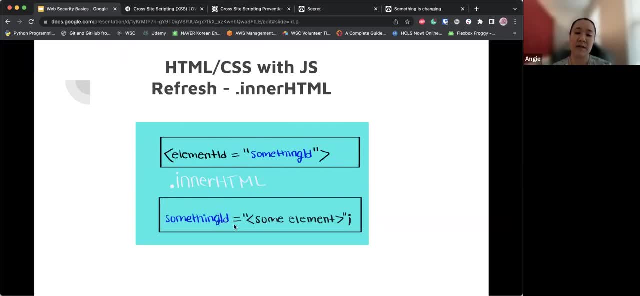 ID and it can be some equal, assigned- excuse me, assigned- to some element there and you have a semi-colon. So this is how they would communicate with each other with HTML CSS, with JavaScript. Just wanted to make that clear before I go further along. Okay, so I have a CodePen example. 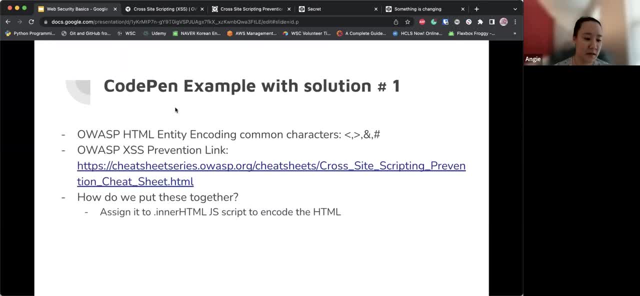 Um, I didn't want to use the typical like VS code and whatnot, and in that example that we're going to do for today, I also want to mention another thing that OWASP has not, not just knowing what XSS is, but how to prevent that, and we can use your HTML entity encoding common. 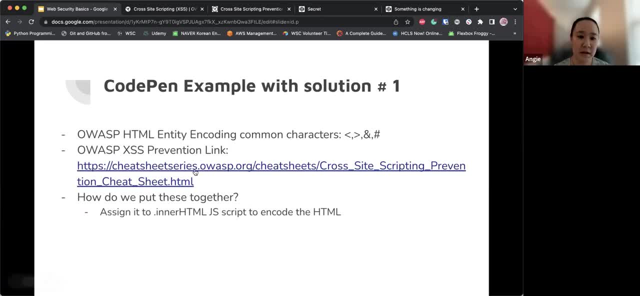 characters. These are a few, but there's a lot and here's a link right here. It's. you can see it right here. I don't know if I can put that in the chat, but this is the link right here. 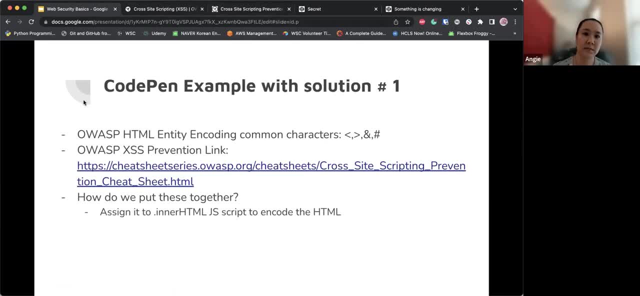 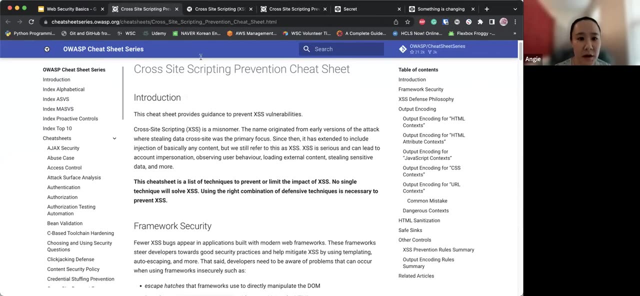 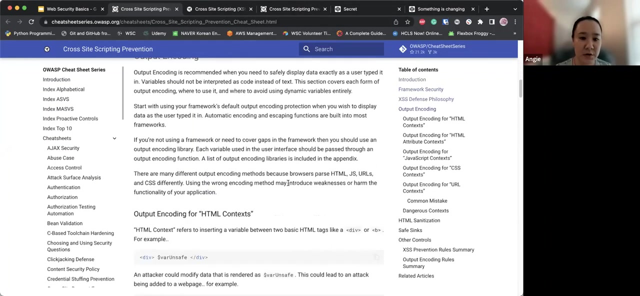 and when you click on this link, okay, what happened? Let me just click on this real quick, Okay, okay, I don't know what happened there. Um, okay, when you click on this link right here, it gives you different types of prevention for cross-site scripting, and I'm going to scroll. 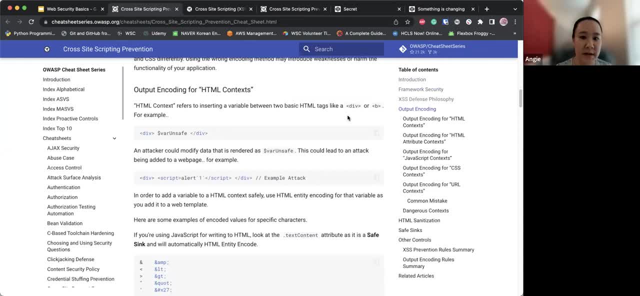 all the way down here. So I'm going to scroll all the way down here and I'm going to scroll down to output encoding for HTML context. So there are things like what I was talking about earlier, like the HTML elements, like div tags or bold tags, and you can use different safe. 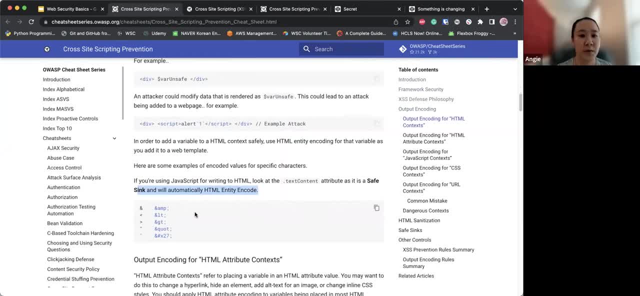 syncs that will automatically encode the HTML, So that script tag that you see here, uh, and ALT or ampersand ALT with the semicolon, and then you can use ampersand gt, the semicolon at that at that part of the script tag, so that way it doesn't. 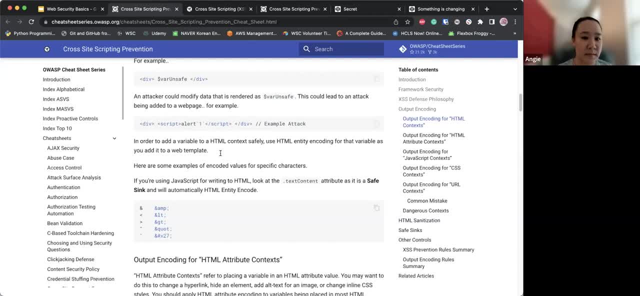 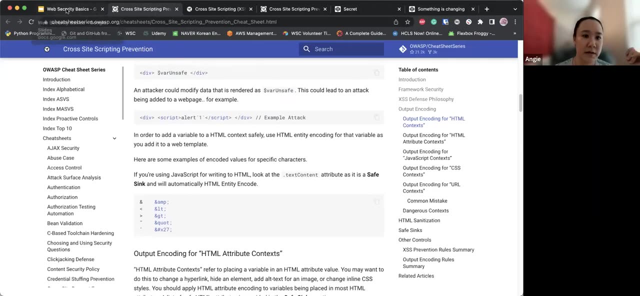 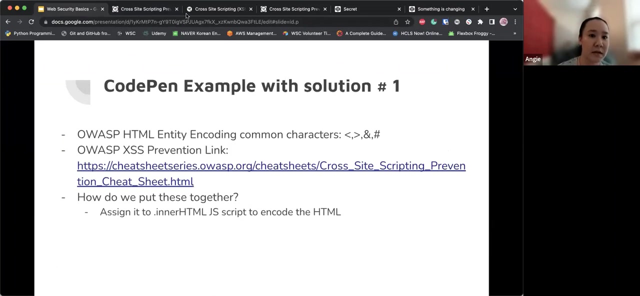 activate when there's some type of attack trying to happen and depending on what else is in the div tag or other html tags you you can use, like the dollar sign and etc. okay, let me go back here see if i can go to the actual um. um, sorry, i'm trying to figure out why i can't find that one codepend link. 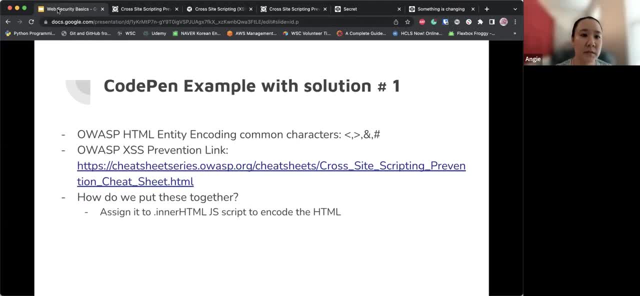 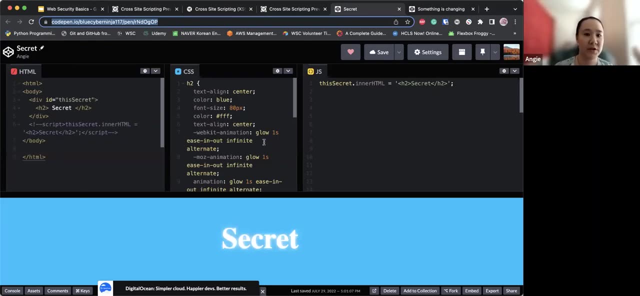 let me see if i can just bring this down a bit. okay, okay, i now i can see it. okay, sorry, i now can see what's going on. so this is the example that i want to show what i mean by the html element with javascript, and for this example i want to use 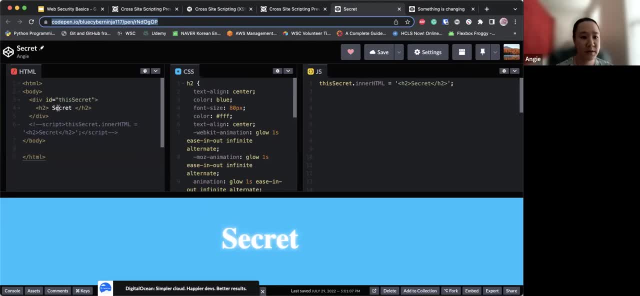 the h2 element or heading to element secret. as of right now it looks like some random plain old heading to, but there could be a script inside here and for those who don't know again how, um, like the text editor or co-editor, even with codepend, how these editors work, the script tag. 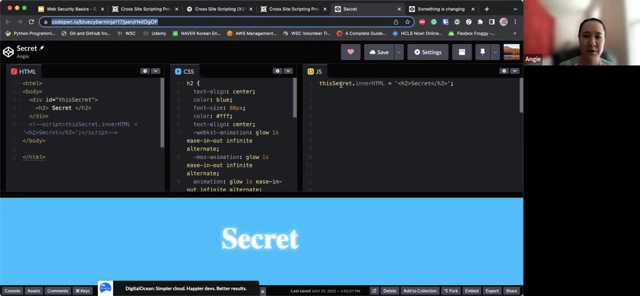 is the same thing right here on codepend and other ones where you have like a dot js file. just want to make that clear. um, so when you have this script tag, it's going to communicate right with div id equals the secret. so this secret right here, that's what we assigned. we gave like a little. 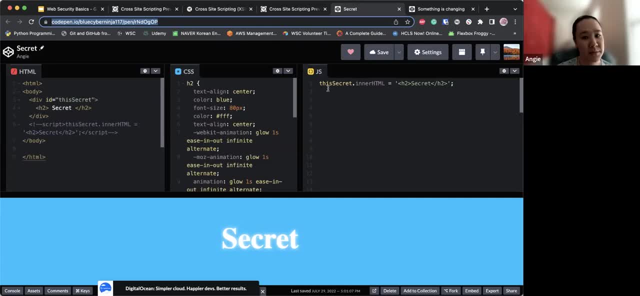 name for the div and we put it right here, which is the same part right here, and we use dot inner html and we assigned it to the secret tag. so this again, this is this can be malicious, like i was saying earlier, because you can put whatever you want inside with inner html. it could be something else. 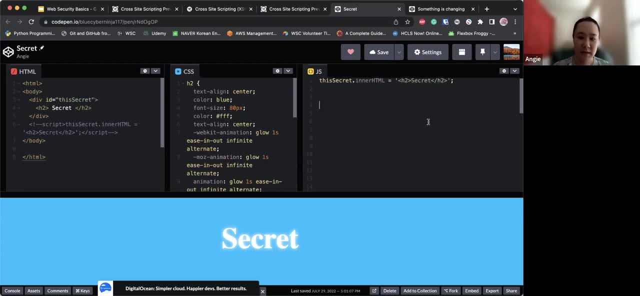 besides this. so how do we mitigate with this example again, we can use the um oasp, uh, the and um lt, and then the and gt, and we can even use a slash for escaping things in javascript, so this can get or set html inside the element. that's what i mean by inner html and i'm gonna 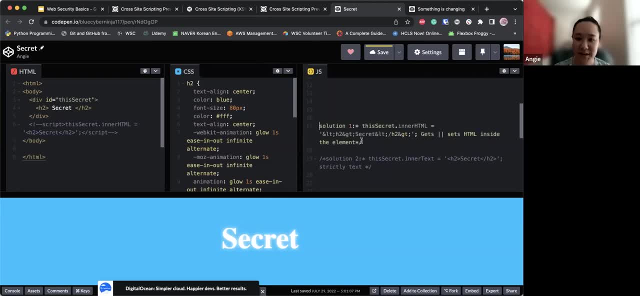 um, uncomment this because i just didn't feel like typing typing this today. so when this is activated, the secret tag should be: oh, hold on. this will drastically change, so it's going to look more like a text. it's going to be encoded. so, as of right here now you can see that it's encoded. it's no longer, it's still the dot. 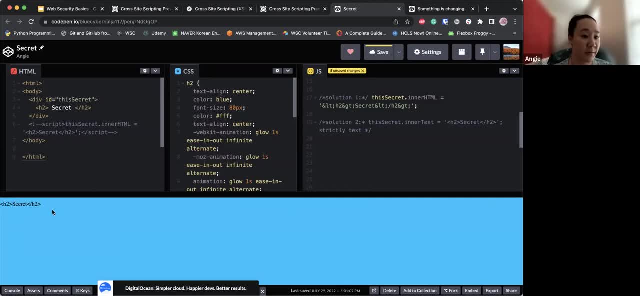 inner html, but we stopped cross-site scripting from happening there by following oas um xss prevention sheet. yeah, so you can also do this in the browser with um web dev tools such as, like, i think, chrome dev tools or firefox. whatever browser you use, and when you encode with this, you can also see what like this actual text too, as output. 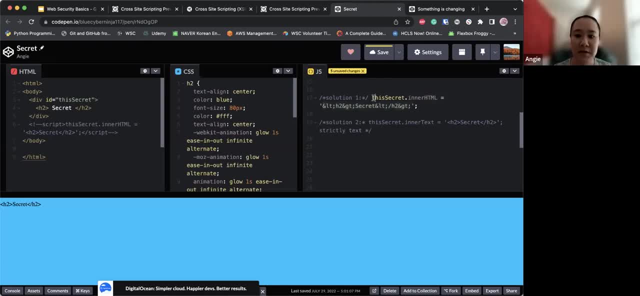 when you're using javascript, and obviously you can make a function with this. it doesn't have to be just one little line, but i just want to make it really simple and easy for beginners, for those who have not been exposed to javascript. so that is. it is possible to still secure the website, so i'm gonna comment this one out. 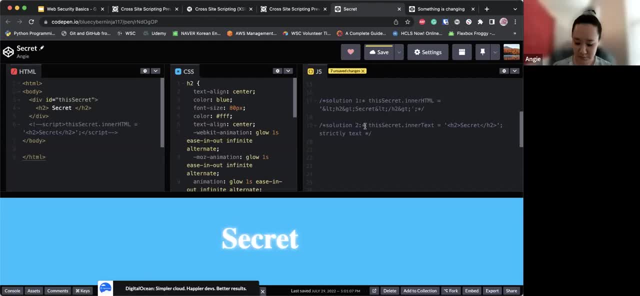 and i'm going to use the second solution here too, with dot inner text and before i show what the output's going to be. the reason why: um, it's safer and a better way to use iter dot inter text over dot enter html's, because this will be just strictly text, it will not be some link that somebody can possibly click on it. 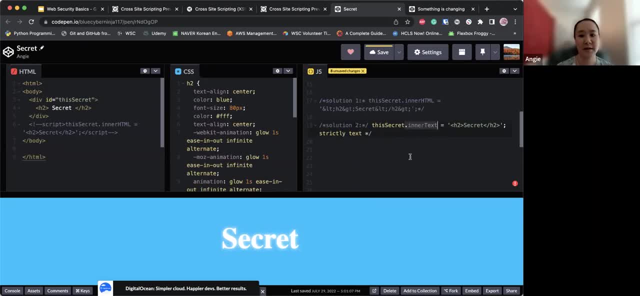 could be some type of xss or cross-site scripting attack, so it's a safer and more secure method. highly recommend that, and i'm going to also comment this out, because keep forgetting to put a lot of comments on this. so when you see this, it will also be the same. but again, this is just text, so 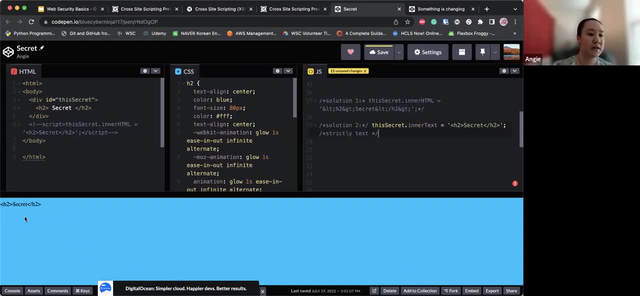 it's going to stop all that input that's going in within the heading two tag secret. okay, yep, so that's one example of how we're using html entity encoding with javascript. the other example that i have is a step further than what this is going to be. 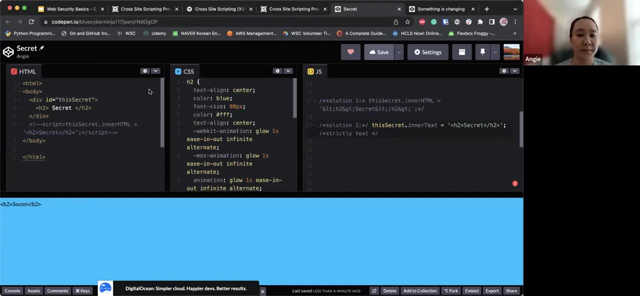 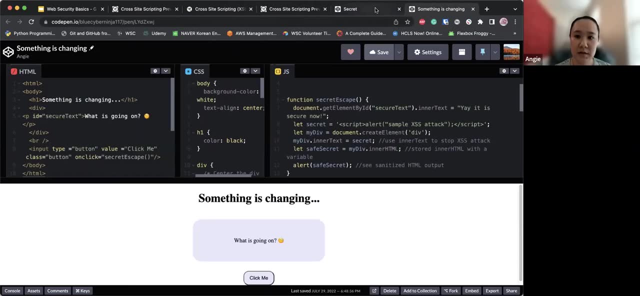 and you'll see what i mean when we get to the next example. let me click on this one here. let me bring this up. sorry, i didn't realize it was out of place. okay, no, i clicked on the wrong one. okay, okay, okay, this is the one i need to look at. 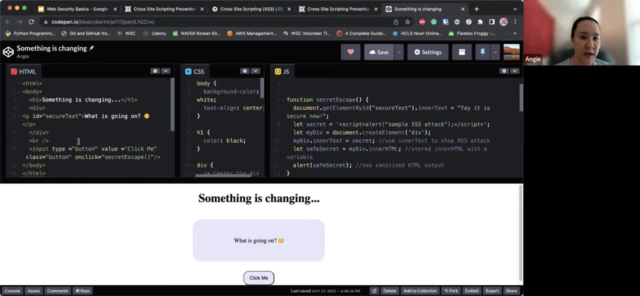 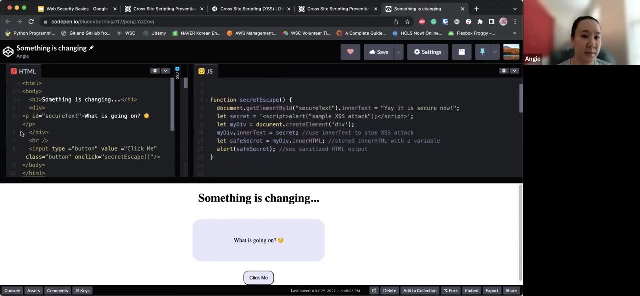 okay. so with this example here, this is a whole lot going on. i'm going to close the css, because this is not the point of the lesson. um, again, we're going to be using the id secure text and this time it's going to be in a paragraph tag. so, like i said, you could not, you could, but. 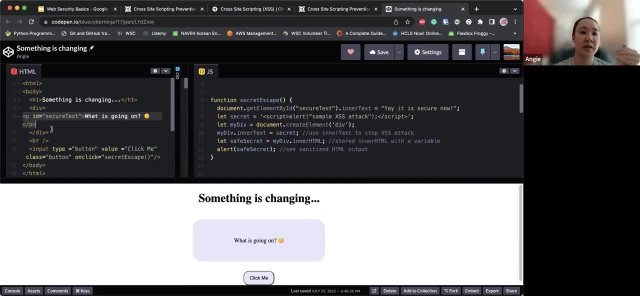 anybody can, especially like the attackers or malicious users. they can put anything that's going within the paragraph tag and do some malicious things. so in this scenario, something is changing, something's going on. what's going on? when you click something, something could happen like an xss attack. um, i made an error. 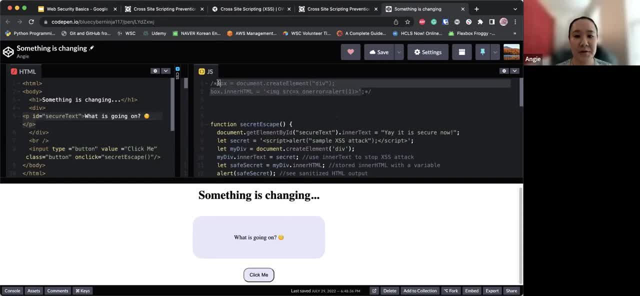 earlier and i commented out, but again, this was another example of cross-site scripting. so when you would click on click me, this would happen. it would come up with a new script and then it would come up with an alert message and it would bring some on error alert and it would delay the website. 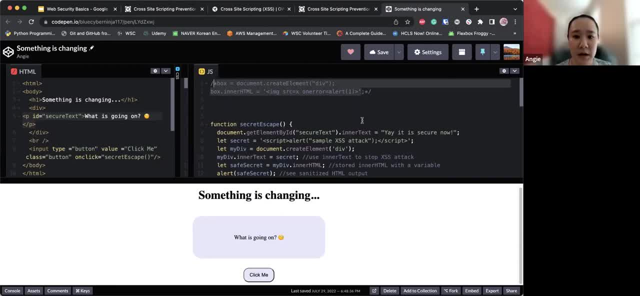 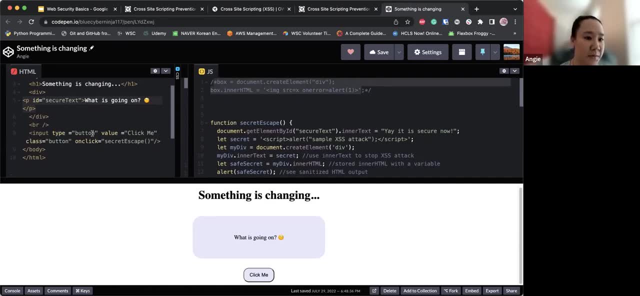 and that's not good, okay. and then another thing that we have going on is something called input type button and then click me and then class button on click. this is key here and it's with the function called secret escape. so the function that we have here. 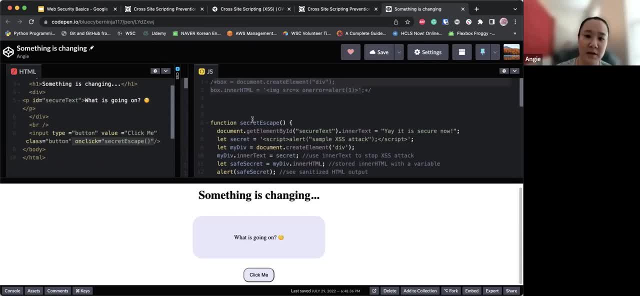 and, by the way, for those who don't know what functions are in javascript or in programming languages in general, it's pretty much a place where you can store all the code that you want. that will make whatever you want it to do, such as, like um, storing variables doing decision making. 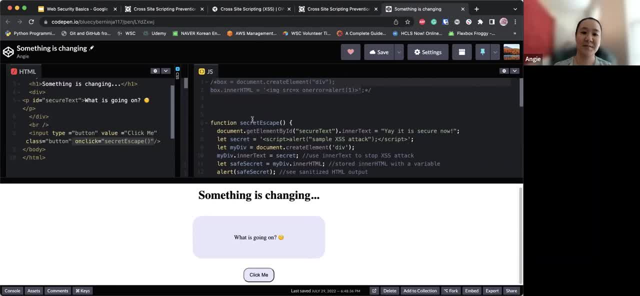 if i'll save it's all that jazz. i'm not going to get into the like the whole like javascript lesson with that. we have more lessons with women who code front end, so but i just wanted to give a little bit of a shout out to the women who code front end, so i just wanted to give a little bit of a. 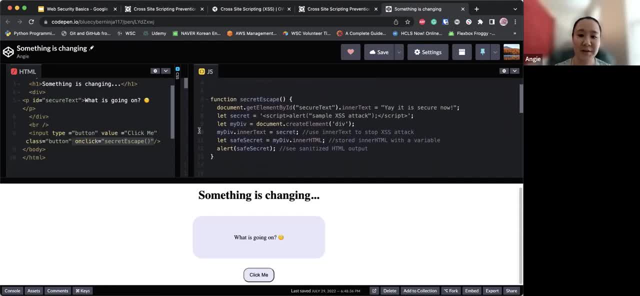 disclaimer, because just wanted to make sure everyone knew what's going on. so we have this function here, with secret escape and the reason why i coded it this way, and it's not just the traditional way. again, there's more than one way to solve the problem. um, i want to use documentget. 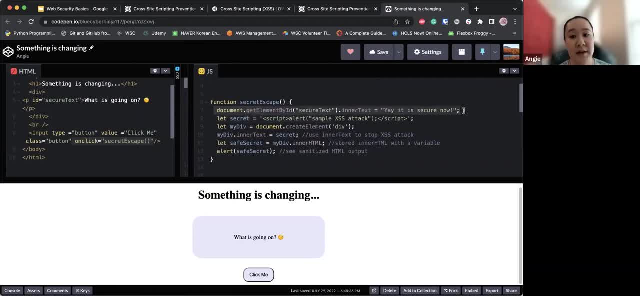 element idsecuretextintertext, like we were saying before, because intertext is one of the best things you could use. i just want to show that this site is secure. um, that's not the problem there. the problem here is within this function. there's some type of script alert. 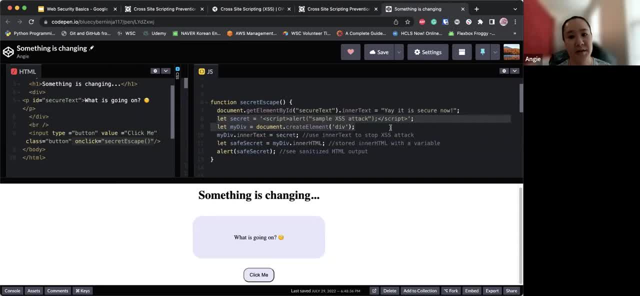 that could. in this scenario it's a sample existence attack. i didn't want to do a real one because i'm not trying to have the whole website hacked and whatnot, so i just want to make a little text that says sample xss attack for educational purposes and what i did with the secret thing. 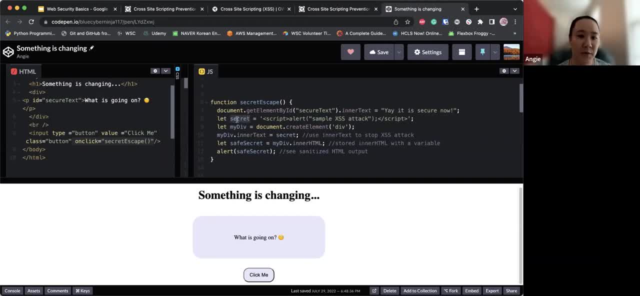 uh, the secret variable. excuse me, i use let because that's what most um javascript developers use nowadays, and they use also bar, but let is the more popular way it's. there's a lot going on with that. i'm not going to get into the details with let versus bar, but we 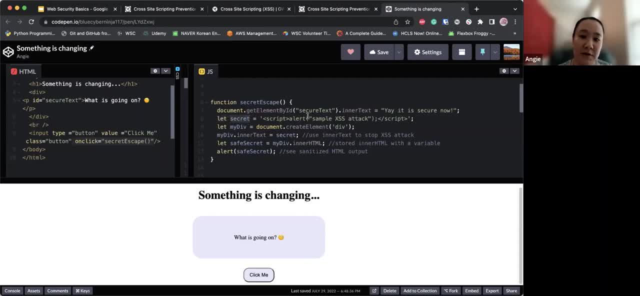 assigned it to a variable called secret and we stored this script here so you can, as you can see, you can have like script tags within script tests within script tags, and whatnot. and then we assigned um, my div, because it was with div, we created a div element and and then we used intertext. 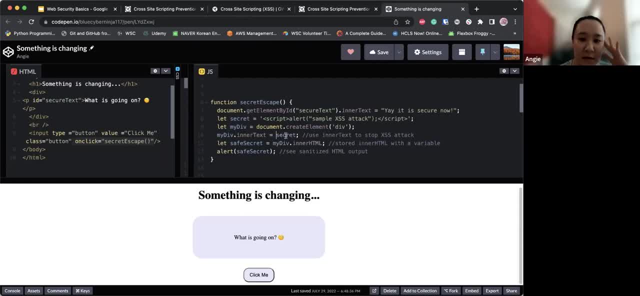 and we assigned it to secret. so we were storing this variable with a div that we made in secret and we just used that to stop the um, the xss attack, and then for educational purposes again. i just want to use another variable to store what was here, because i wanted to show that. 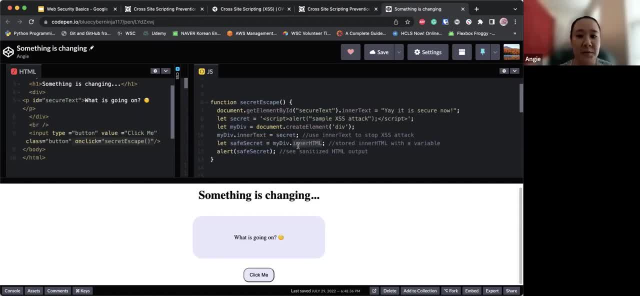 you can still use inner html, um, because it's used actually a lot in javascript with within, like the web web development community. so i'm not saying that you should never, ever, use it. just use it wisely and securely. make sure that things are encoded, make sure things that are, um, sanitized, and that's what we're doing. we're. 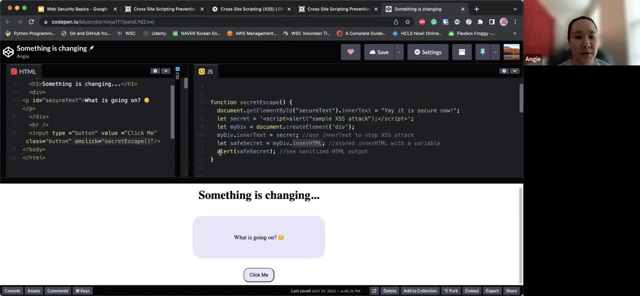 sanitizing things and again, with this example here, i didn't want to, um, just leave anything hanging. i want to show people what that variable did, to show that we actually did some encoding. so when i click on the button- click me, it should show you the code that that variable did, and i'll show you that. 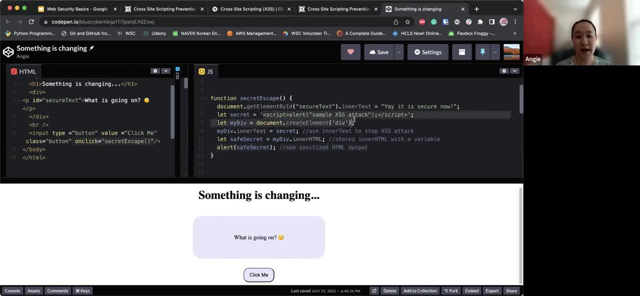 show how this script alert tag- excuse me, this script, excuse me- is, you know, encoded like we use with OWASP, with the and I think, ampersand LT and then and ampersand GLT. 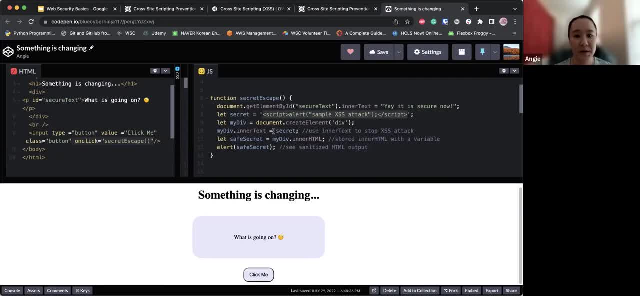 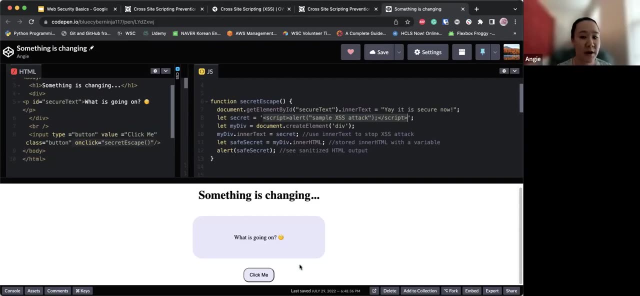 all of that jazz that we saw from the previous example, And then I think that's it for this part. Oh, so also, when you're going to see right here, with what was it? Yeah, secure, test what is going on, It's going to say, yay, it's secure now. So don't get all caught. 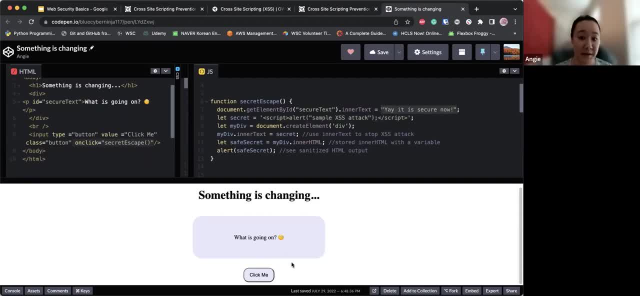 up with that. It's really the click me part that I'm trying to stop the XSS, the button that we had. Okay, so when I click on this, you should see an alert. So what we did here was we stopped the alert and we encoded it. 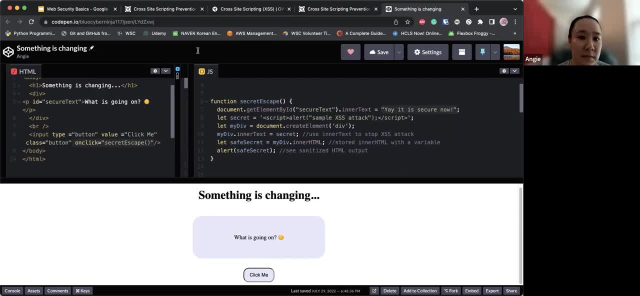 We encoded it by using and LT semicolon script. You notice that it's not activated, because we stopped it by using the HTML and T encoding with JavaScript, and then and GT and then semicolon, and then it still shows this, but it's not doing that. if that makes. 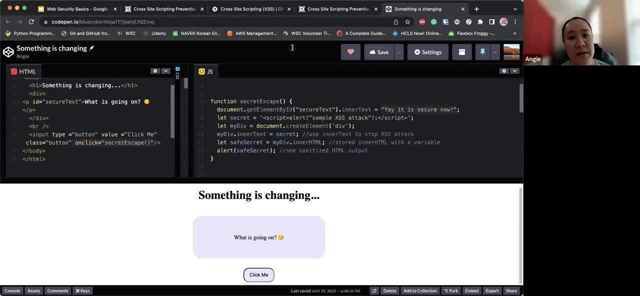 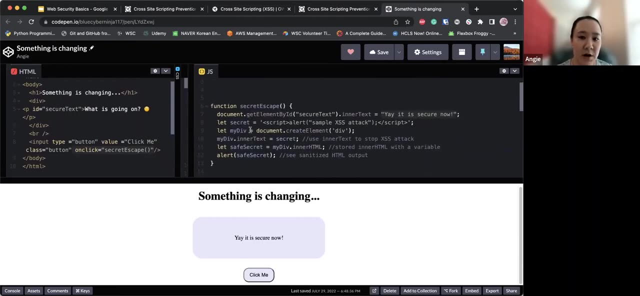 sense It's not doing that attack because we stopped it by encoding it and we did some escapes going on too, with the script Yep. I think that's all I had for the moment. There are another? well, actually I do have. 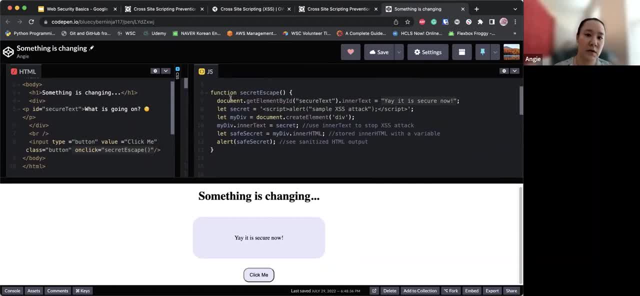 another thing: When you are doing like HTML encoding with JavaScript, you don't have to always write as function and whatnot. You can use like the arrow function, which is more like a one-liner way of securing- not just securing, but of writing what you want. 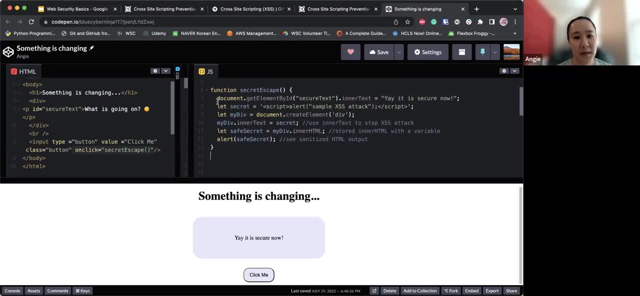 to do with the function. So, yeah, that's all I had. It was just a really basic web security webinar. And well, actually I do have one more thing. I thought about it. So I know that this is for women who code front end. I understand that this is really. 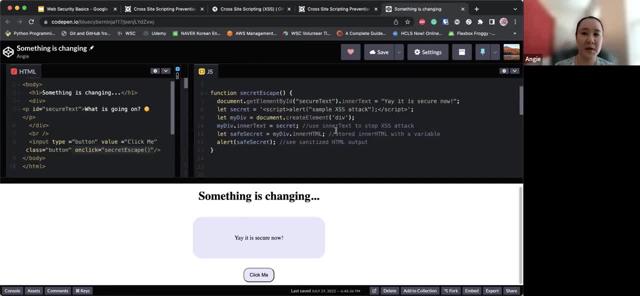 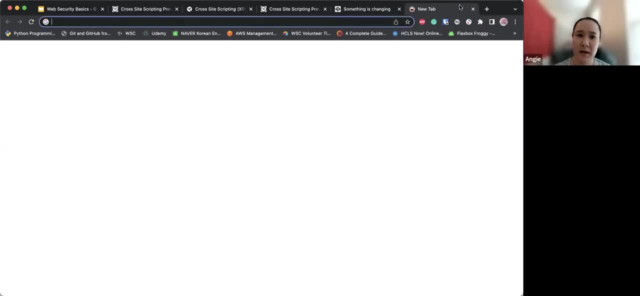 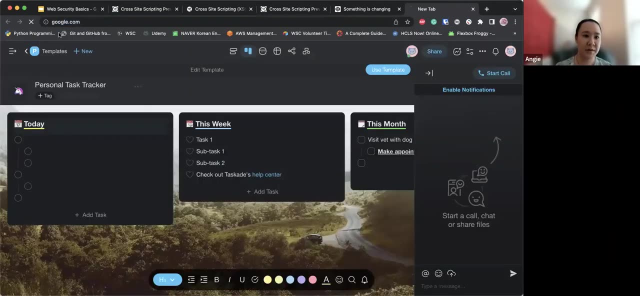 basic of what's going on here. There is something called NPM and I think it's an HTML sanitizer. I don't have the link on me, do I? I think, if I just go to Google and I just type in like: 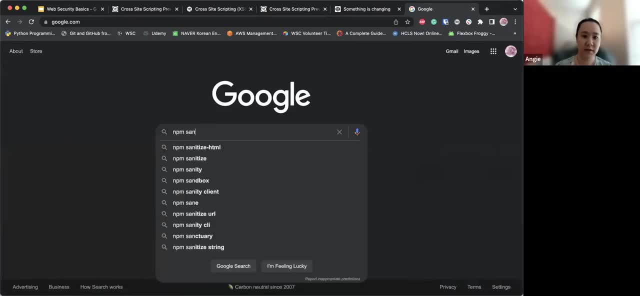 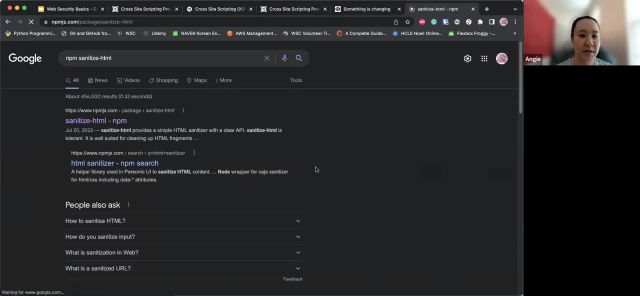 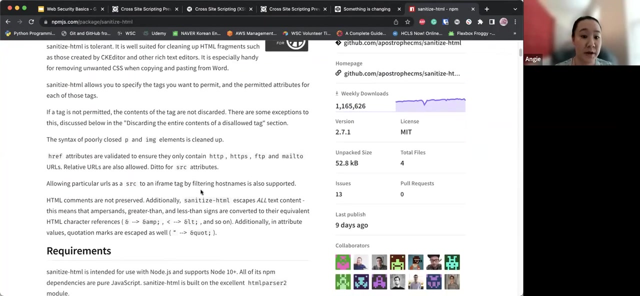 NPM- sanitizer or something like that. it should show up: Yeah, NPM sanitize HTML. So you can use this API if you're just tired of doing the encoding itself and just plugging it in and setting it up. Here's the steps here. And you use TypeScript. 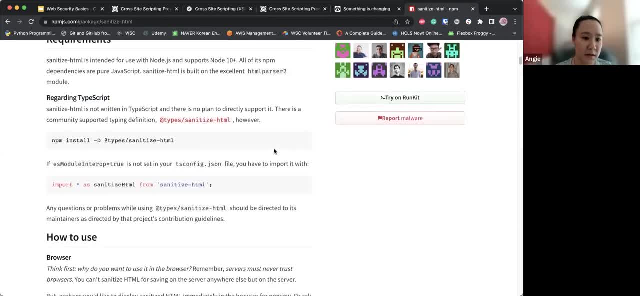 Okay, All right, And there's all these different instructions. There's more than one. So if you don't want to just do HTML encoding with JavaScript manually and you feel like you want to be cleaner and smoother with that, you can use APIs as well. 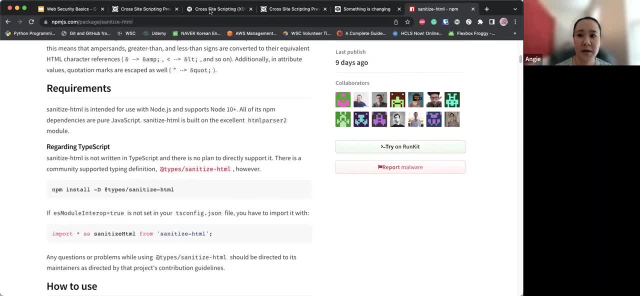 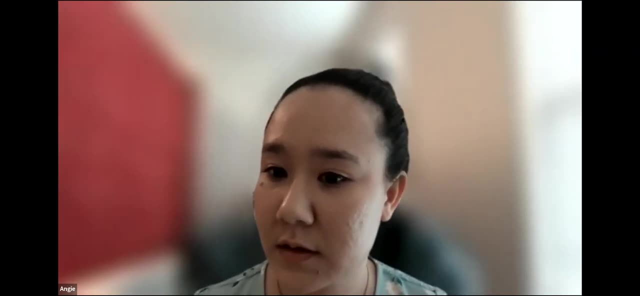 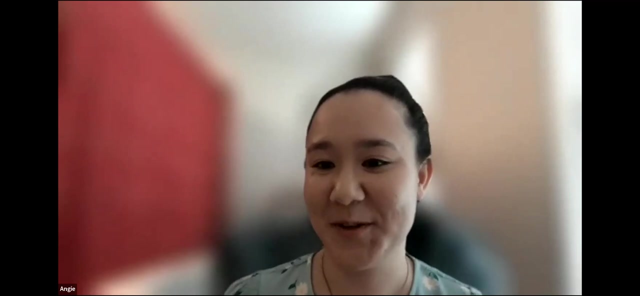 So that's all I had on my end, And now we can have questions and whatnots. Okay, All right, Let's see if we have any questions. Thank you, Does anyone have any questions on the presentation? I know it was really short, but just wanted. 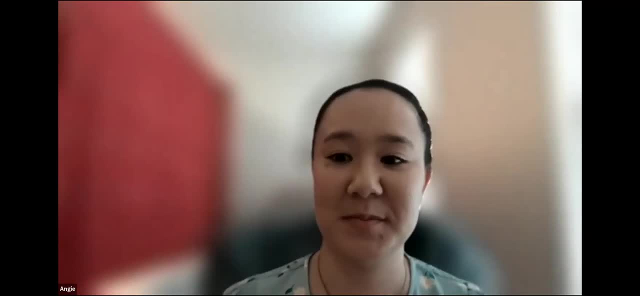 to make it as simple as I could. I know there was many people from different backgrounds and I wanted to make sure that everyone was able to hear When it comes to like web development. I have actually a little bit to start with. 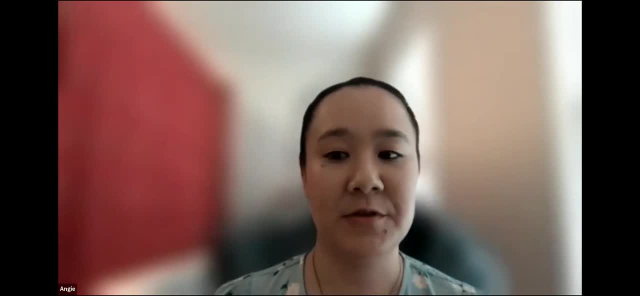 that too. Like when I first started Women Who Code, I was actually not really doing a lot of coding myself. I had a lot of imposter syndrome. So I want to also give a shout out to Stephanie for encouraging me, as well as our other fellow. 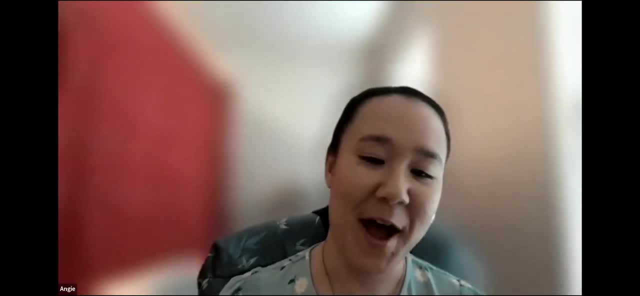 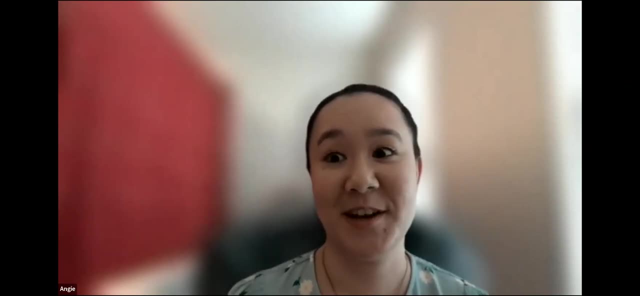 even with Women Who Code- friend Princea, I believe, is how I said her name- for also encouraging me to do web development. So yeah, I highly recommend Women Who Code, regardless whether you are a beginner or advanced, or in between. 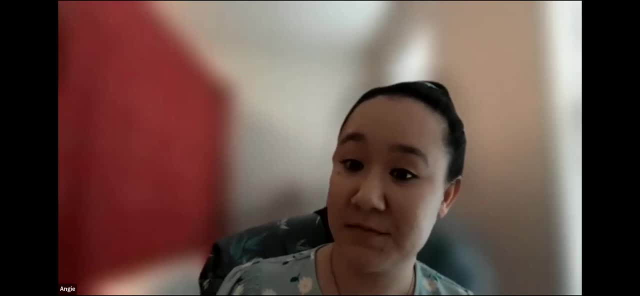 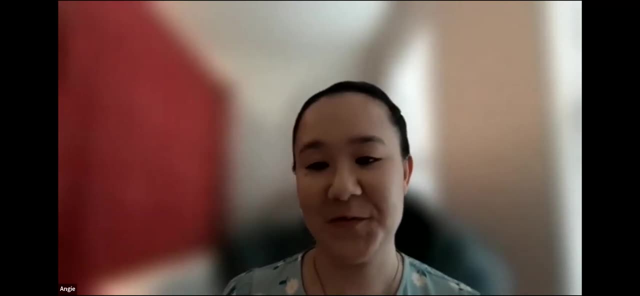 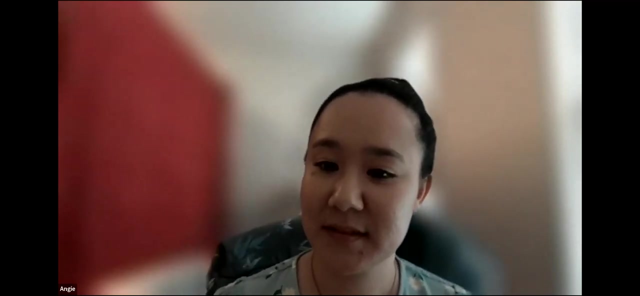 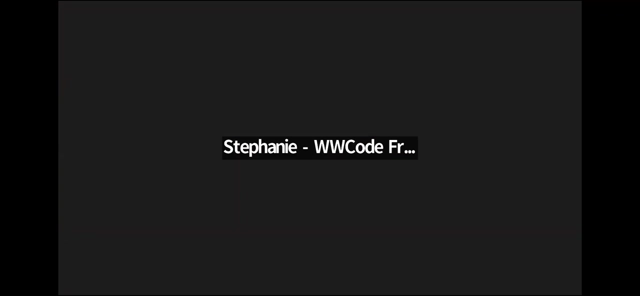 Yeah, you can do that as well with regex Yep. Yeah, I didn't mention that for today because I didn't want to go further and further. but yes, you can do that as well. There is one question in the Q&A. Could the developer ensure the input only accepts text and not HTML or any other scripting language? I haven't looked into like other scripting languages such as Python, but I know for a fact that there's something out there that has like some syntax. 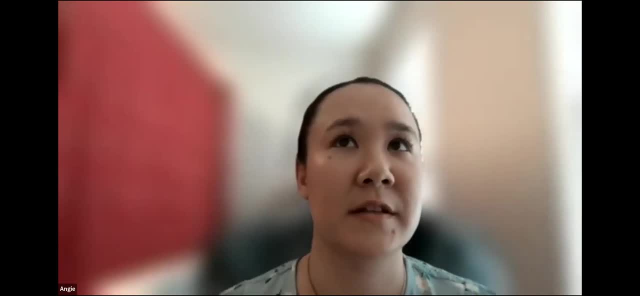 Yeah, Yeah. Yeah, That's a good question. I don't know if Python can do that. Yeah, I think there's some sanitizer like API of some sort, like with Python, I think, or Java- I can't recall on the top of my head, but definitely through like a Google search. 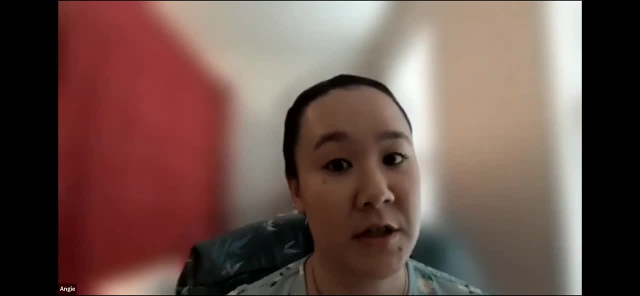 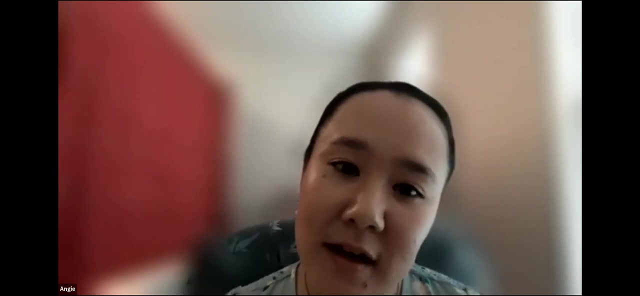 or you can actually do it manually, like we did today, like making a function of some sort by using some text, intertext. Okay, Let me see. Can you perhaps give an example of your code being personally attacked? I mean Okay. 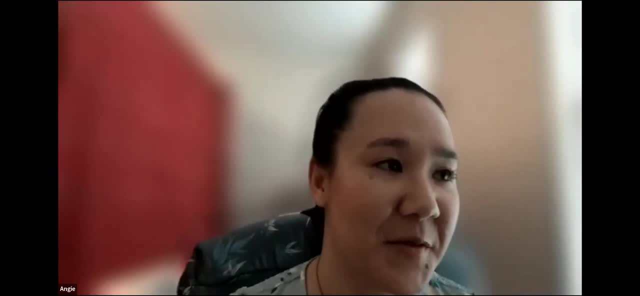 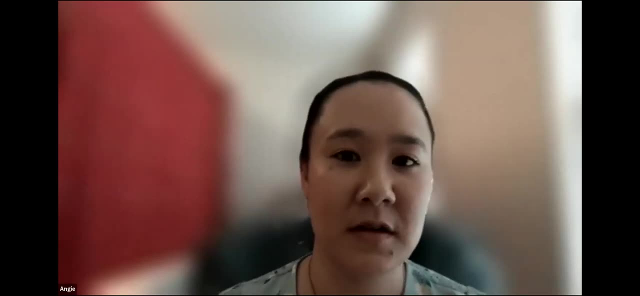 if I took out that one comment from earlier, it will show like an alert message and it had like the number one. And if I were to do that, I mean it's not gonna really mess with that CodePen example, but I just didn't want to take my chances with it. Obviously, we could sanitize it by using 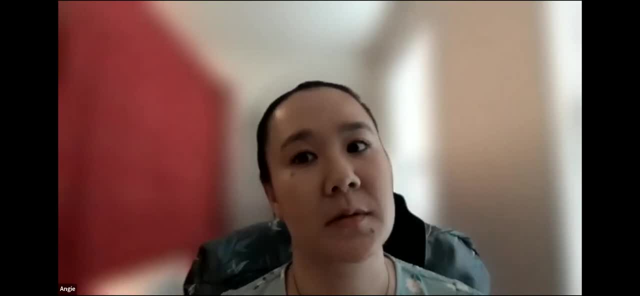 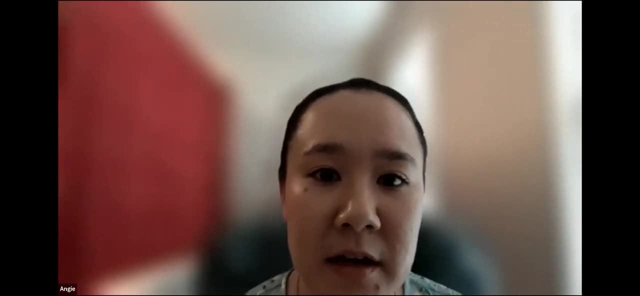 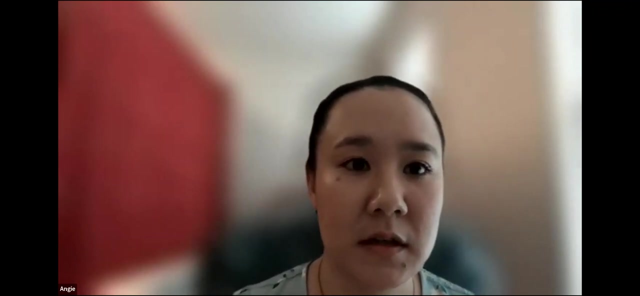 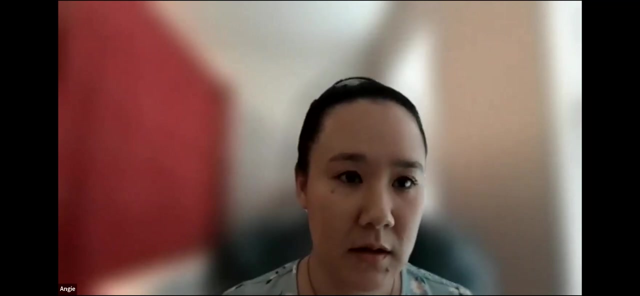 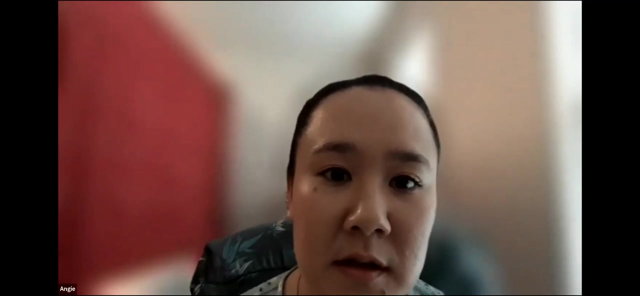 the OWASP methods in place or using like an API. Oh sure, I can share the links, Let me share the OWASP ones. That was XSS, So this one's going to be with the prevention for OWASP. Okay, Let me see, So it has one. ensure the server sanitizes the script when it receives. 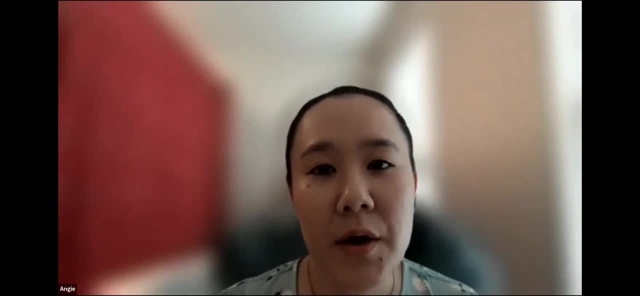 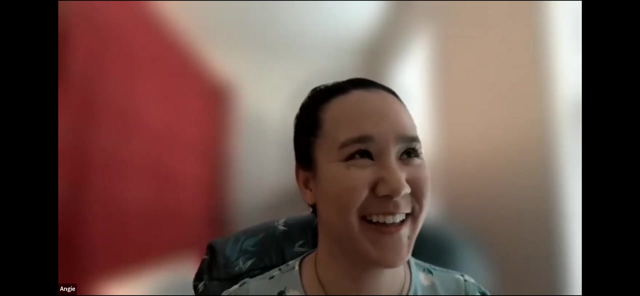 or to fight the cross side. Okay, So you're not talking about, like the manual, what we did with the functions and whatnot. The API should communicate with the server, Like if you're using, for example, NPM. I don't know why I struggled with those letters. 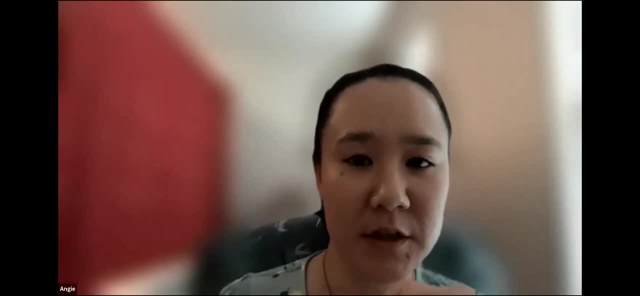 NPM, It should help. I haven't installed NPM or like the HTML sanitizers just yet because I ran out of time earlier this week, But if you were to install that, it should give you some type of like output, that like some type of message. There we go. 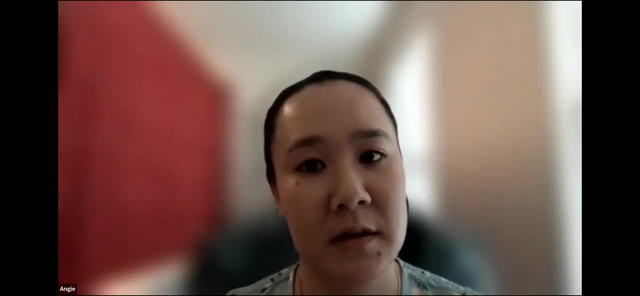 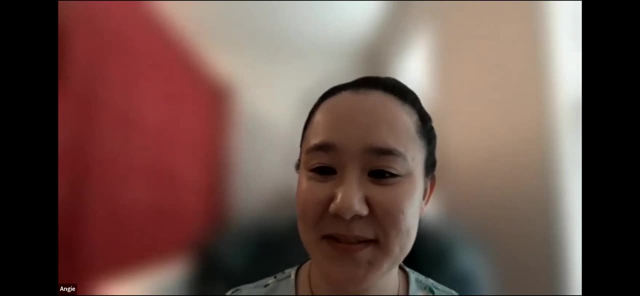 That will show that it's going to fight against the cross-site scripting. Maybe that could be for another webinar. People are up for that. Are there any other questions or comments? Oh, awesome, Thanks for joining. I don't know if there's any other questions. from what I've seen, 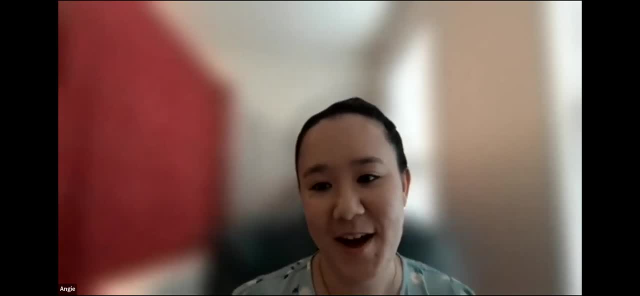 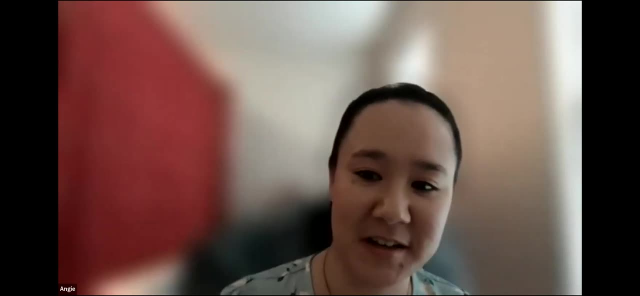 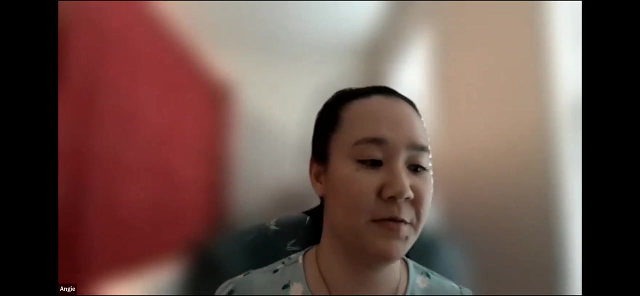 Okay, Let me see. Oh nice, Oh, Joanna's here. Awesome, You're welcome, Claudia. Thank you so much. Yeah, Like I said before, I definitely recommend Women Who Code. regardless of where your path is in your on your coding journey, You will learn a lot with us. I can definitely recommend that, And 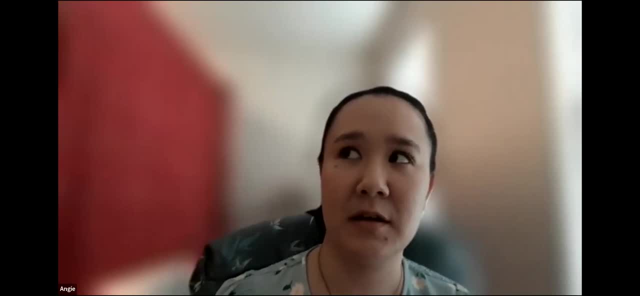 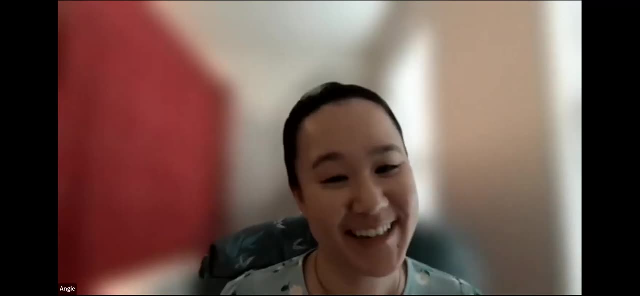 I think there's some. we definitely have, I think, monthly events or weekly events, depending on what track you're in. I know, for Women Who Code Python, there's a lot of activity going on there, And then now I think there's like a JavaScript study group too for Women Who Code. 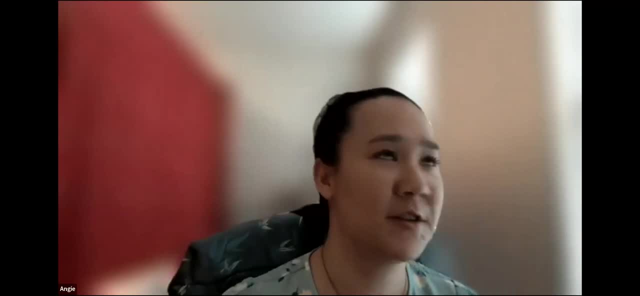 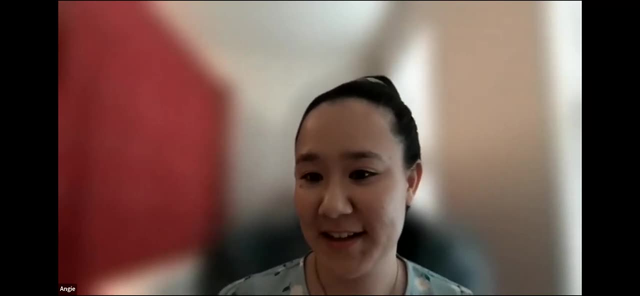 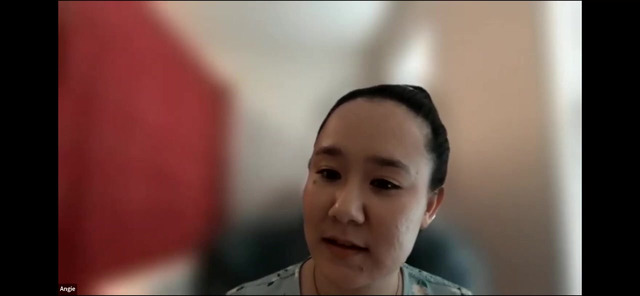 and it's called Women Who Code, Frontend, And I think there's one for data science. There's so many different ones. So yeah, just start showing up and you'll learn a lot. You're welcome. I just realized did I even send you guys- the excuse me, you guys, the everybody- the NPM link? 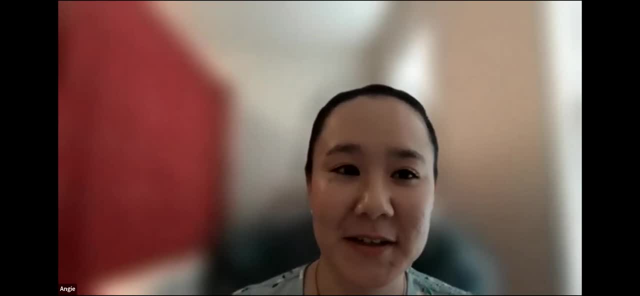 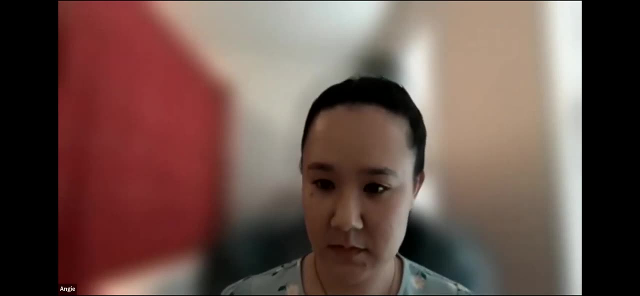 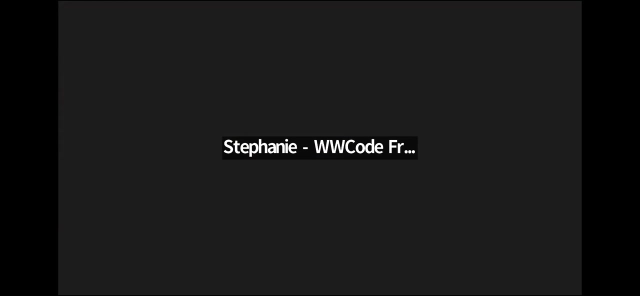 I don't even know if I sent that, Just realized I didn't send the NPM link. So that was one example, like I said earlier, how you can sanitize your HTML. We also had another question in the Q&A from Mark: What happens when the cross-side script executes? Can the server defend against it? If so, how? 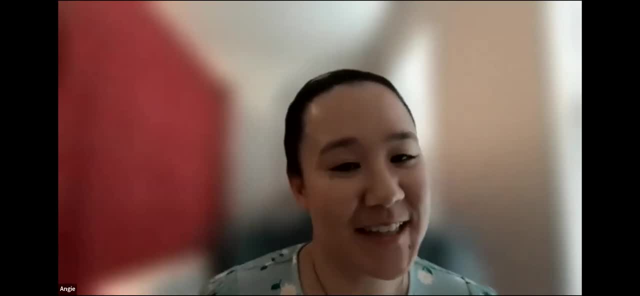 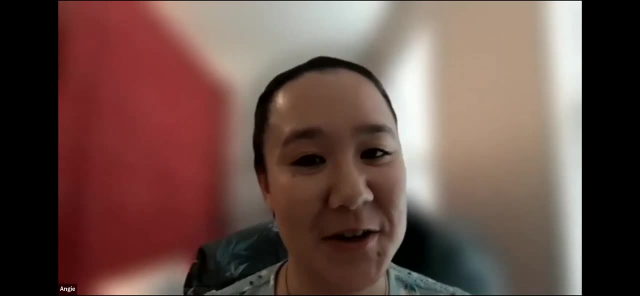 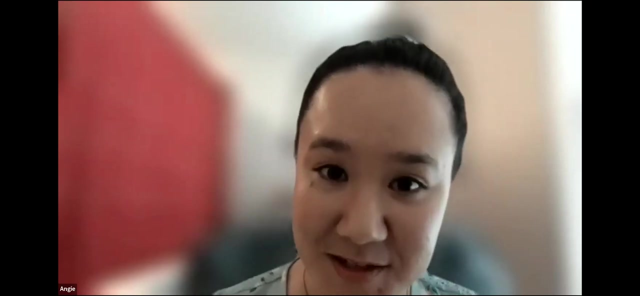 Okay, so this is a little bit above what's going on Today's event. this is where I know where this is going. This is with the security question: Yes, if there's security policies in place, and if not, find some ways to mitigate that by including some security policies. 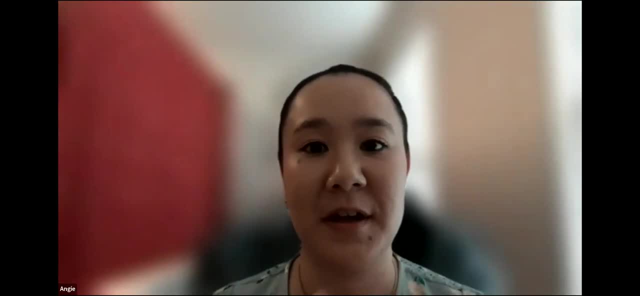 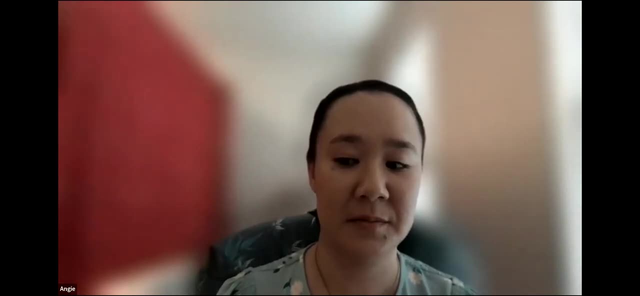 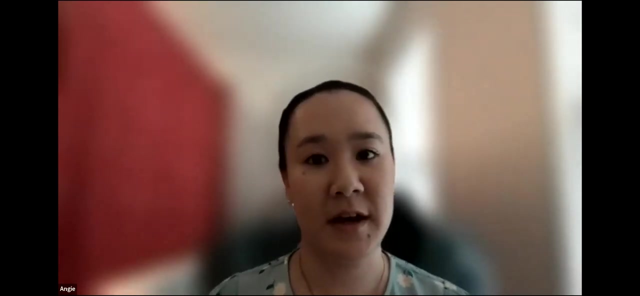 That also is like with the communication thing going on, that security analysts, even developers, should communicate, because one of the first things that goes on within the security world- whether you're on the web developer side or security analyst side or a manager side- 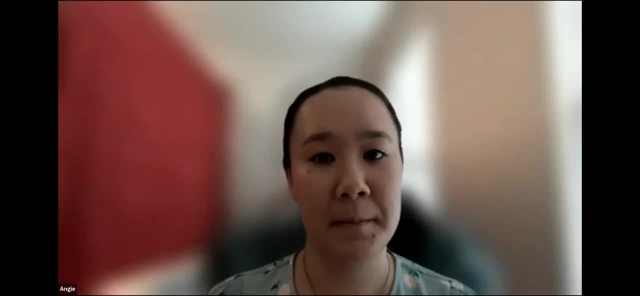 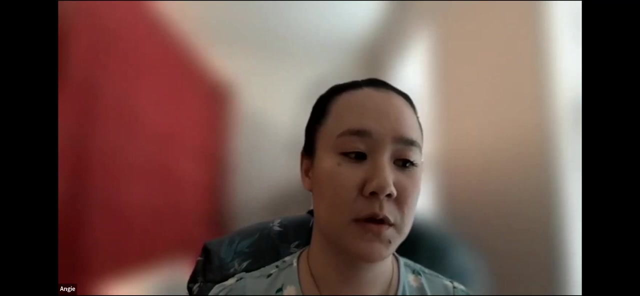 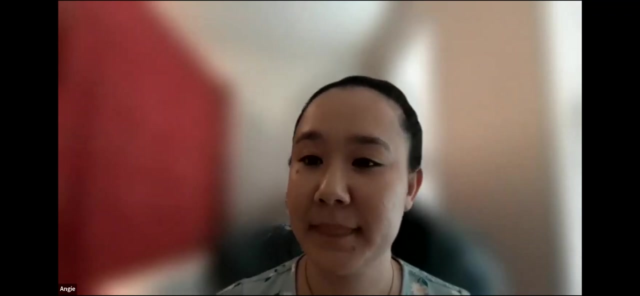 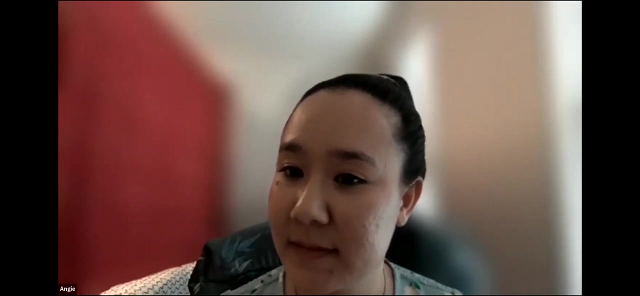 talk to each other, figure it out, come up with security policies such as using the OWASP, because they are a web application security organization and they offer many resources of how to include, like potential cross-site scripting attacks. So that, again, is where we would want to help you know. 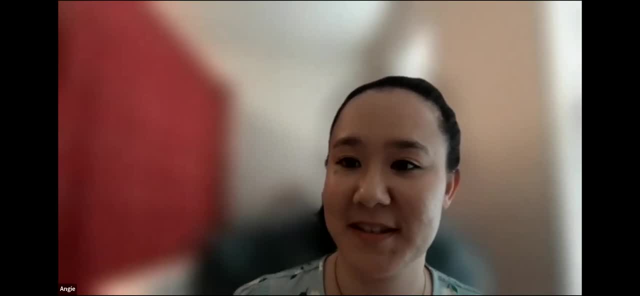 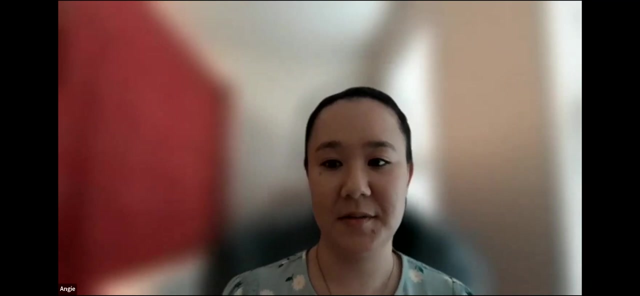 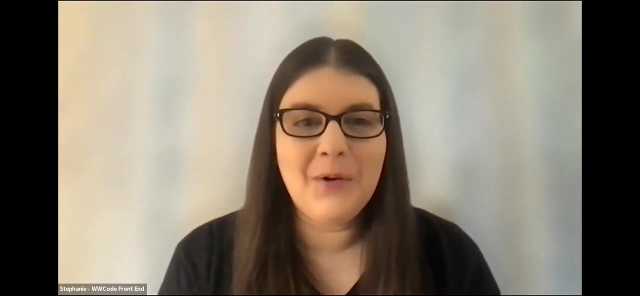 Are there um any more questions or comments? Mark, is there any other questions or comments? Okay, awesome, All right, fantastic. Well, that was an amazing talk, Angela. Thank you so much for joining Women Who Code Front End today to deliver this insightful webinar. 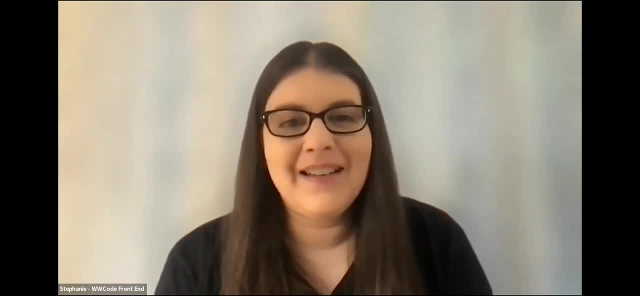 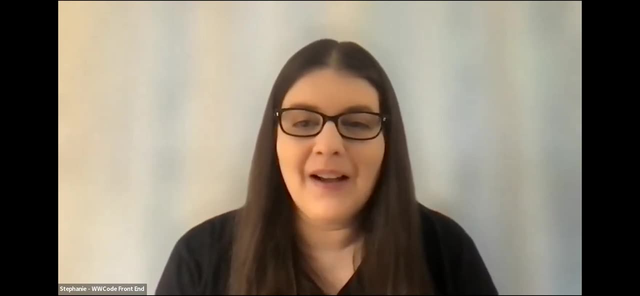 We really appreciate it and amazing, amazing job, And thank you everyone so much for attending today. You were a wonderful audience and this was an awesome session. Thank you everyone so much for engaging, And I did share a link to the womenwhocodecom.